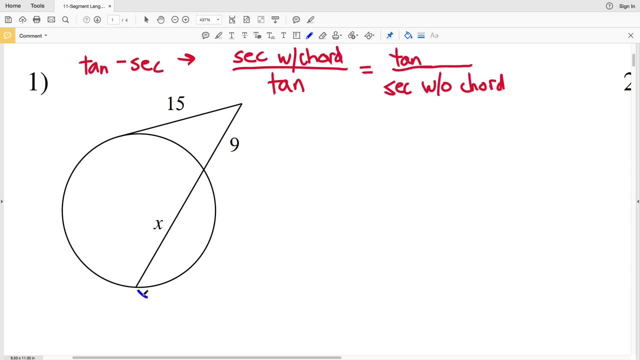 So in number one setting this up, the secant with the chord is this entire length, which is 9 plus x. So we will have 9 plus x all over the tangent length of 15.. That's going to be equal to the tangent length of 15 all over the secant without the chord. 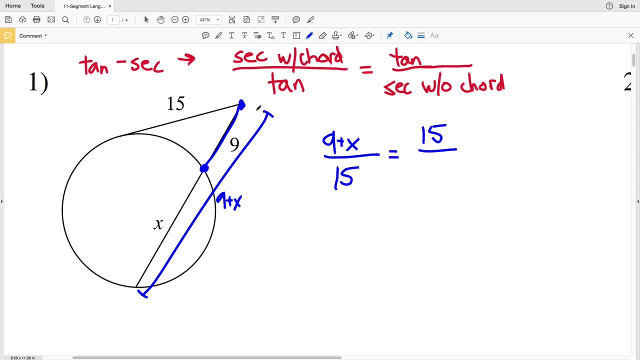 and if the chord is x, that secant length without the chord is just 9.. So now we're going to cross-multiply and solve for x, multiplying 9 plus x to 9 and 15 to 15.. So 9 times 9 plus x will equal 15 times 15.. 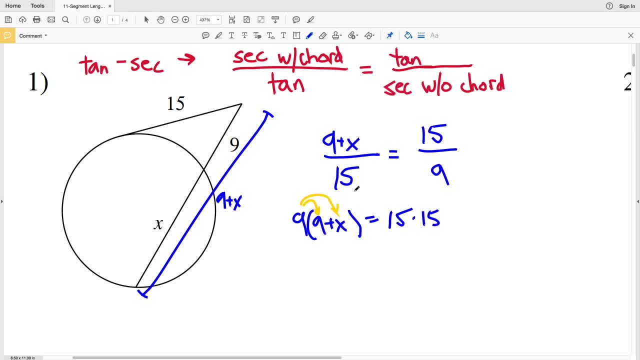 So I'll distribute the 9, and that will give me that 9 times 9,, which is 81,, plus 9x, 9 times x will equal 15 times 15,, which is 225.. Now I'll subtract 81 from both sides. 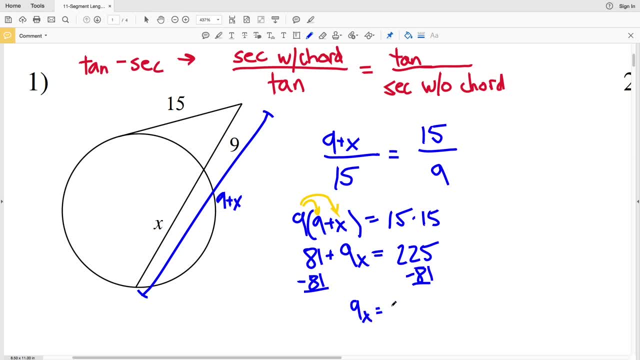 In doing that, I'll get that 9x is equal to 225 minus 81,, which is 144.. And my final step will be to divide by 9.. 9 divided by 9 is 1.. 1 times x is x. 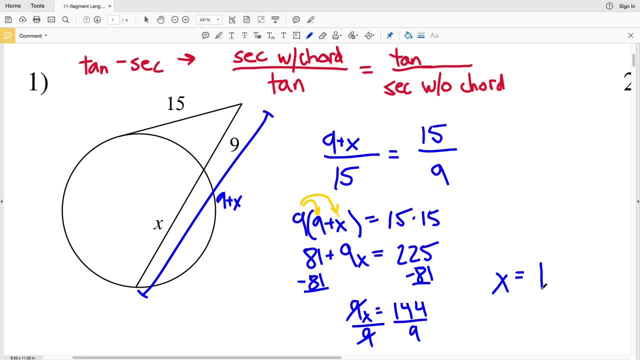 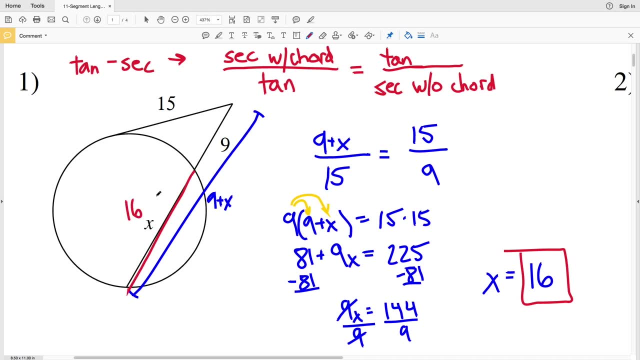 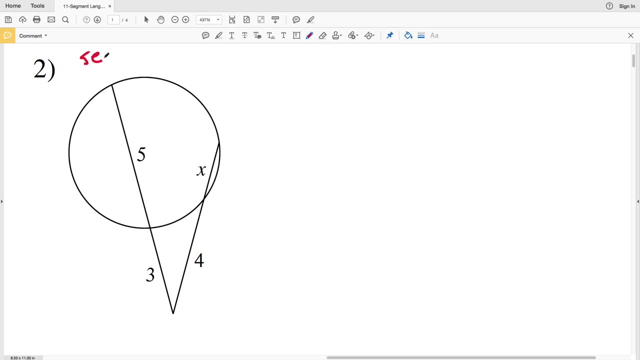 So x will be equal to 144 divided by 9, which is 16.. So that segment length x is 16 in number one. Now in number two we're going to be using a different formula, because this time we have a secant and a secant. 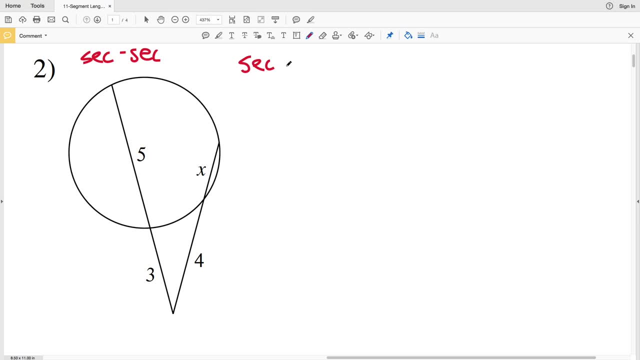 So that formula is that the secant length with the chord, so including that chord, so the entire secant length times the secant length without the chord, will equal the secant length of the other line with the chord times the secant length. 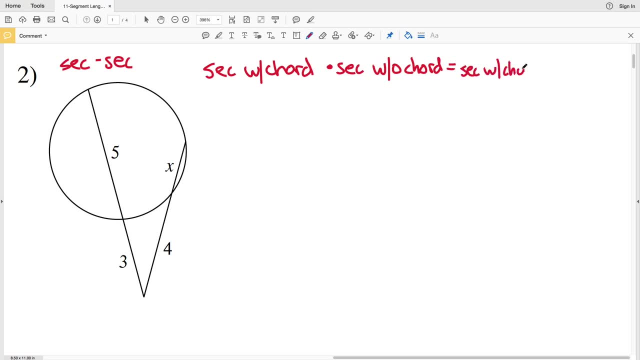 of the other line without the cord. so again the secant. so let's look at this first, three and five. so the secant with the cord will be three plus five and if we're multiplying that to the secant length without the cord, that would be multiplied to three. that's going to equal this other secant. 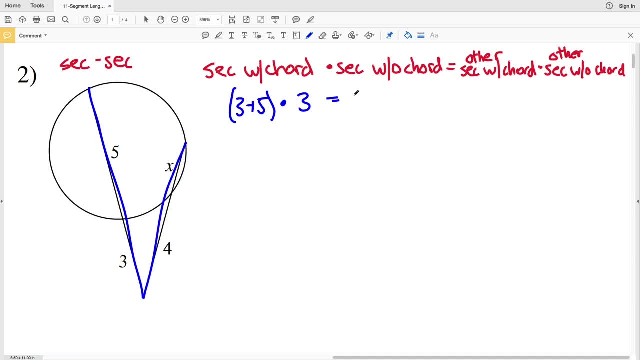 so that length with the cord, so the entire secant length four plus X times the secant without the cord, that would just be four. so essentially we're taking the whole secant length of one segment and multiplying it by that external secant length or the external segment that makes up that secant. 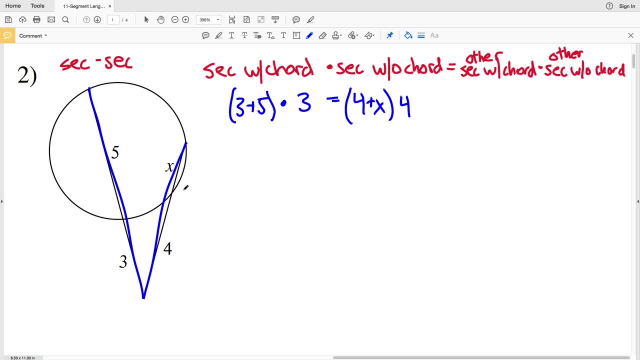 and that's going to be equal to the other secant. length times the external segment of that secant. and so I'm going to distribute my four and I'm going to simplify on my left: 3 plus 5 is 8, so we'll have: 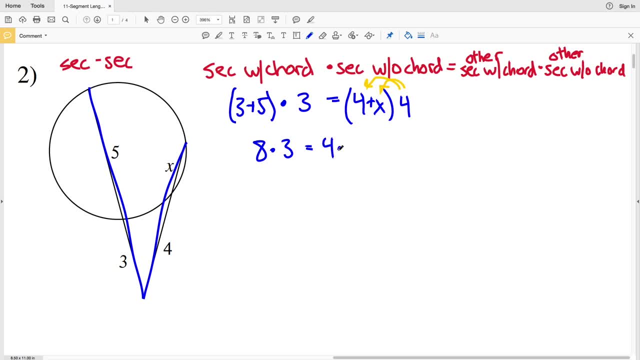 8 times 3 equal to 4 times 4, which is 16 plus 4 times X. 4x 8 times 3 is 24, and that will be equal to 16 plus 4x. so now I'll subtract 16 from both sides to get 8 equal to 4x. and when I divide by 4, 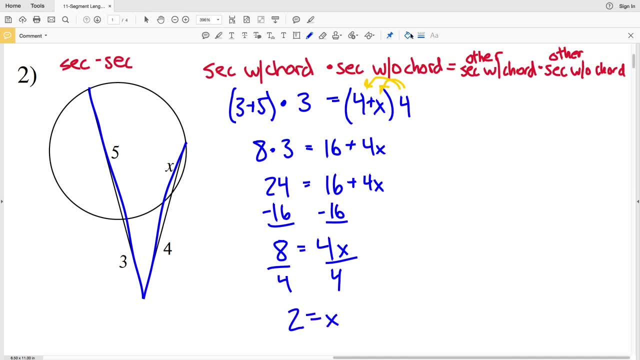 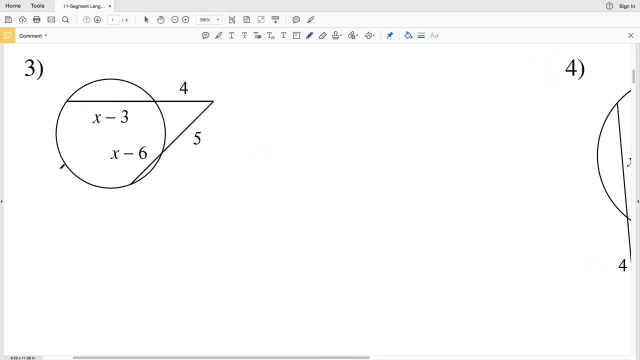 I'll get that 2 is equivalent to X, so 2 is my solution and number two and number three. I have another secant, secant intersection where I'm finding the segment length, so it'll be the entire secant length. looking at this top secant line, 4 plus X minus 3 and we're going to be multiplying that by that external. 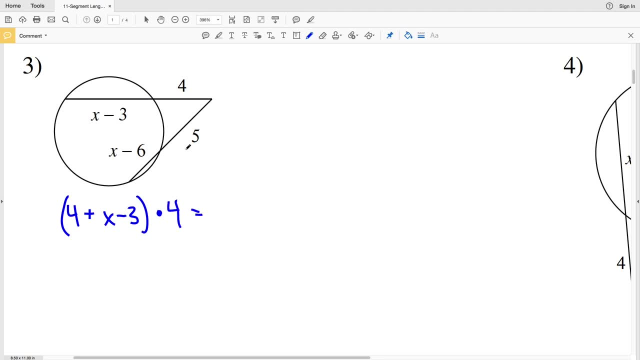 length of four, that's going to be equal to the entire length of the other secant 5 plus X minus 6, and that quantity will get multiplied by that external length of 5. so before I distribute the 4 and 5, I'm going to combine like terms. so I'm going to combine 4 and. 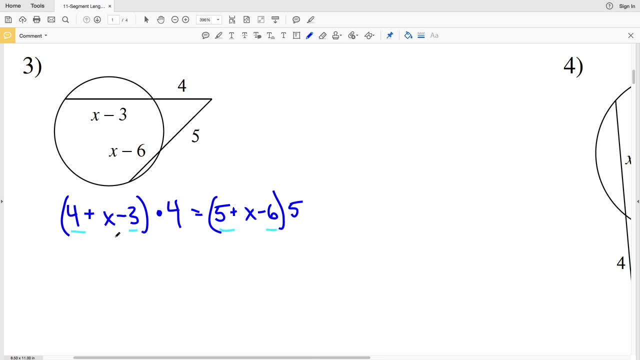 3 and 5 and 6. so 4 minus 3 is 1, so I'll have 1 plus X. multiplying that by 4 will equal 5 minus 6, negative 1 plus X by 5. now I'll distribute the 4 and I'll distribute the 5. 4 times 1 is 4 plus 4 times X is 4: X. and now 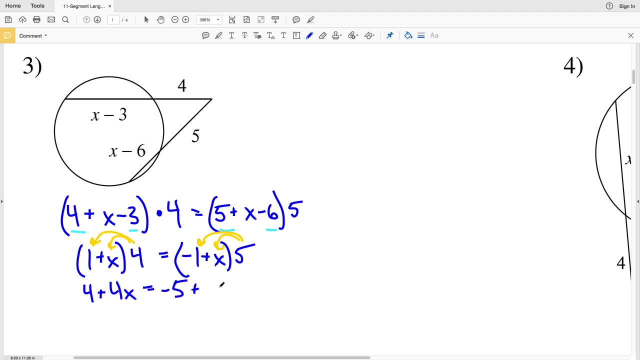 we'll be equal to 5 times negative 1, which is negative 5, plus 5 times X, which is 5, X. I'll subtract 4x from both sides, moving my terms with X to the right, and I'll add 5 to both sides moving. 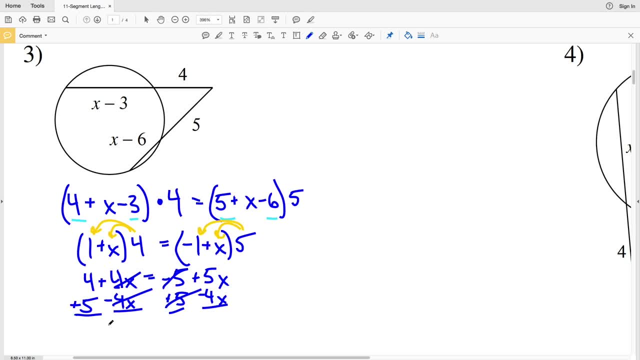 my terms, without X, to the left-hand side of my equation. so 4 plus 5 is 9 and that's equal to 5 X minus 4 X, which is 1 X or simply X. so number 3, 9 is our solution. a number 4 I'm dealing with a. 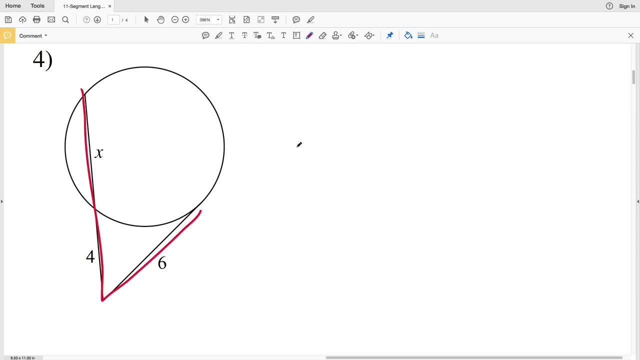 secant line and a tangent line. so, remembering our formula, that's the entire length of the secant. 4 plus X over the tangent line, 6 equals to the tangent of 6 over the secant length without the chord. so just this external length of 4. now I'll cross multiply. so 4 times 4 plus X will equal 6 times 6, and 6 times 6 is 36. so 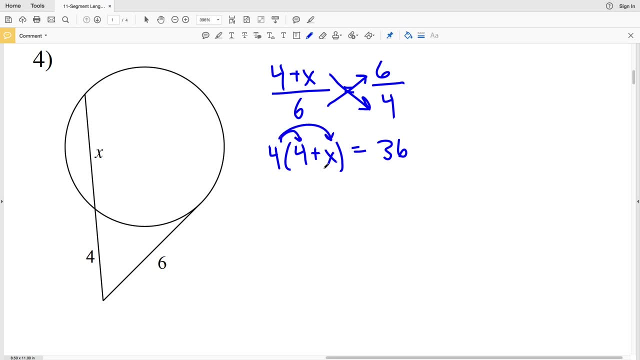 distributing my 4, 4 times 4 plus 4 times X: 4 times 4 is 16 plus 4 times X is 4 X, that's equal to 36. so when I subtract 16 from both sides, I'll get that 4x is equal to 20. and finally, dividing by: 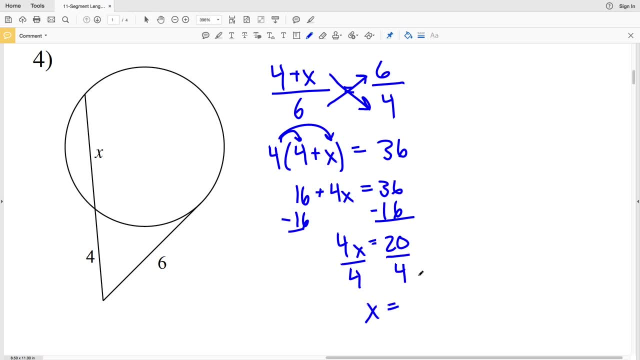 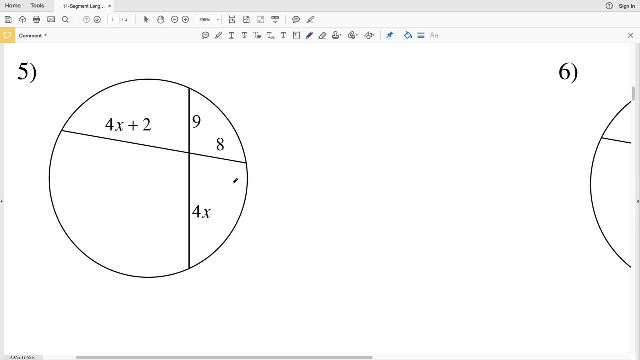 4, I'll isolate my X, and that will be equal to 20 divided by 4, which is 5. so 5 is my solution. in number 4- now number 5- I have an intersection of chords, so my intersection occurs within the circle. therefore, I'm going to be introducing a new formula, so the intersection of chords is going to be. 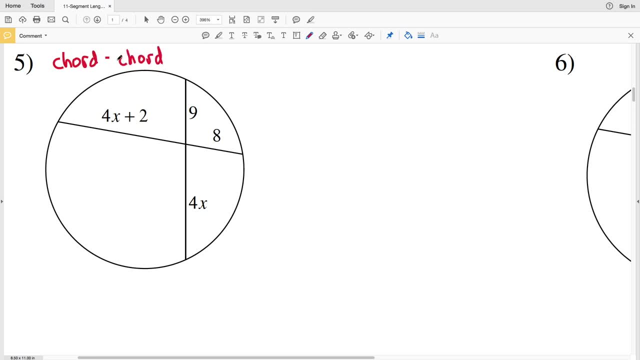 the intersection of chords looking at the segment length. so this is a chord chord intersection as opposed to a tangent secant or secant secant. this formula is going to be the small segment length of the chord times the large segment length of that same chord will equal the small. 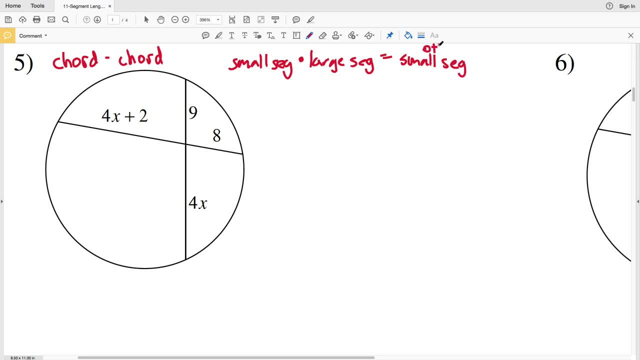 segment length of the other chord times the large segment length of the other chord. so essentially what we're doing is we're taking a portion of the chord up to the intersection and multiplying it to the rest of that chord and then doing the same thing, taking portion of that chord. 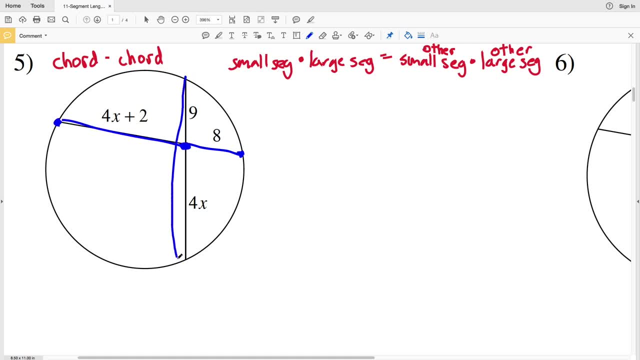 up until the intersection and multiplying it, those will be equal. and remember, multiplication is commutative, so it doesn't matter whether you use the smaller side or the larger portion first. so, looking at number five, looking at this first chord, we'll have the small segment of nine. 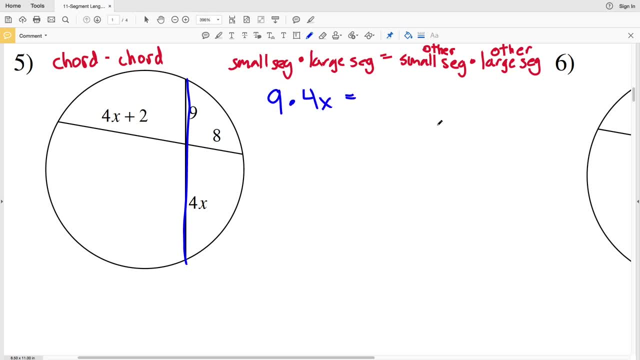 times the large segment of 4x and that's going to be equal to, looking at the other chord- the small segment of eight times the large segment of 4x plus two. so I'm going to have to distribute it: eight on the right hand side and nine times 4x is 36, X and that will be equal to 8 times 4x, which 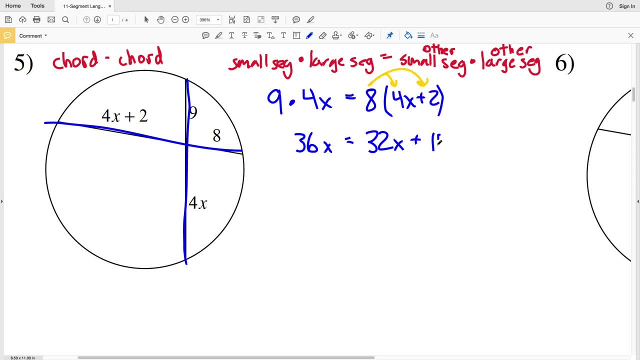 is 32 X plus 8 times 2, which is 16. so I'll subtract 32 X from both sides and doing this, so I'll get that 4x is equal to 16, and simply dividing by 4 will give me that X is equal to 16. 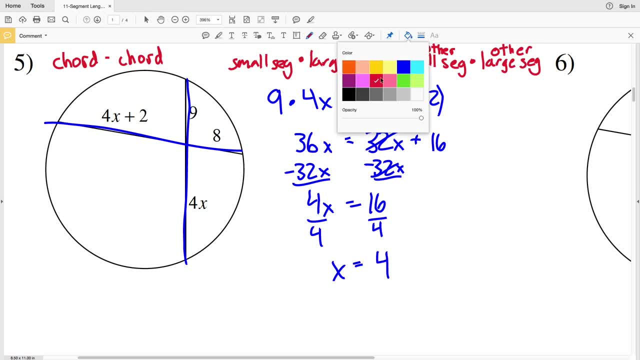 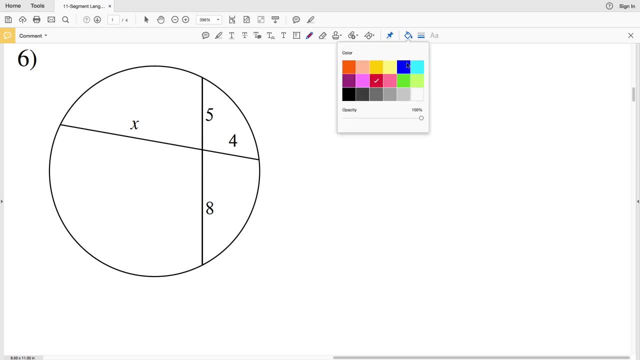 divided by 4, which is 4. so 4 is my solution and number five and number six: again, I have an intersection of chords, so that intersection is occurring on the inside. so I'm going to take a portion of the first chord five times the other portion of that chord, eight. that will be equal to 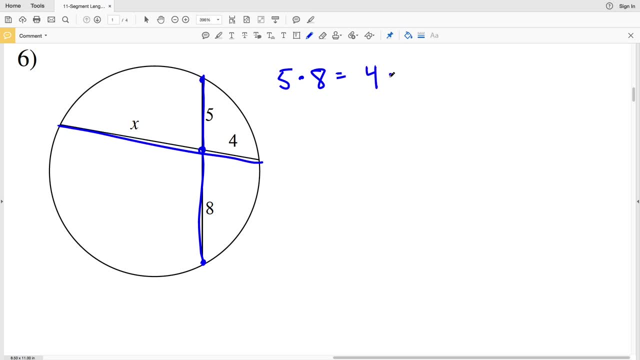 the small portion up to the intersection of the other chord times the other length of that other chord of X. so 5 times 8 is going to be equal to 4 times X. 5 times 8 is 40 and that's equal to 4. 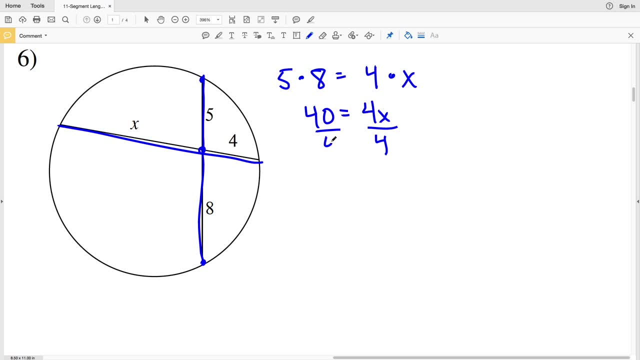 times X, 4x, and when I divide by 4 I'll get that 10 is equal to X in number 6. so if I wanted to, I could plug that value of 10 in for X to get that this segment was equal to 10 and number seven. I have tangent secant intersection occurring outside, so that's. 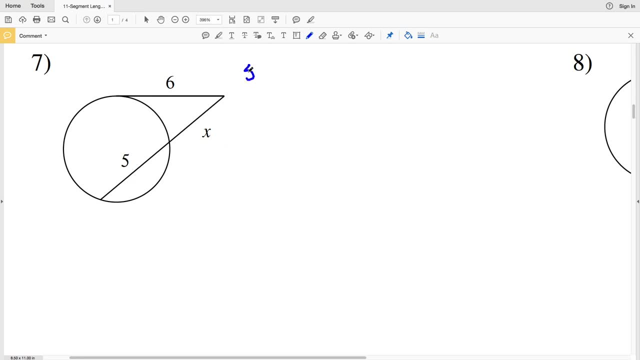 going to be the secant length. that entire length of 5 plus X over the tangent is going to equal the tangent length of 6 over the secant length, without that chord. so essentially that external secant length of X cross multiplying I'll have X times 5 plus X over the secant length of X. so 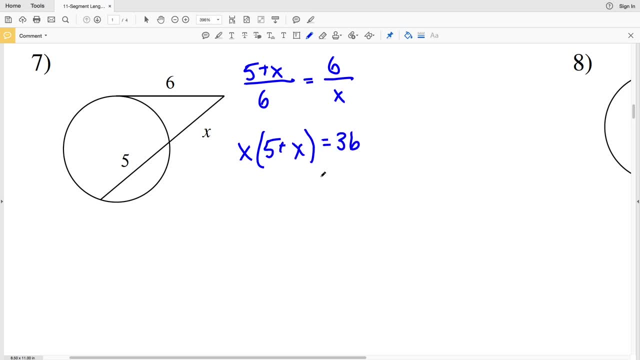 I'll have X plus X equal to 6 times 6 of 36. now I'll have to distribute my X X times 5 is 5. X plus X times X is x squared, and that is equal to 36. now there are a couple ways to go about solving this. 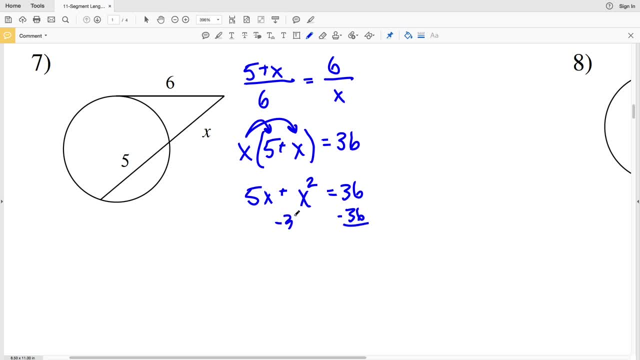 problem I'm going to solve by subtracting 36 from both sides, and then I'm going to rewrite this equation so I'll have X squared plus five, X minus thirty, six or plus, and I'm going to go back to the negative. 36 will equal 0. now I'm going to factor, so what adds to give me 5 and multiplies to give. 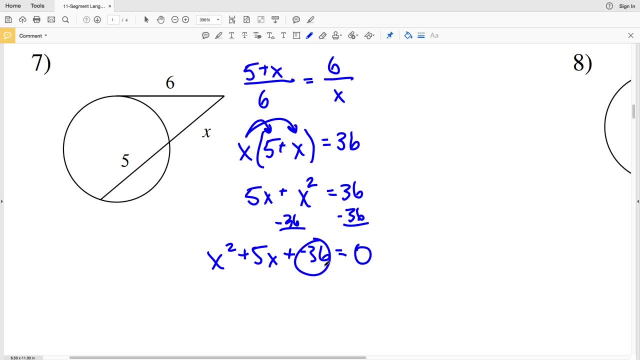 me a negative 36, thinking of the factors of 36, 9 and 4 of both factors, and 9 minus 4 is 5, and 9 times negative, 4 is negative 36, so I'll have X minus 4 times X plus 9, that is equal to 0, so in 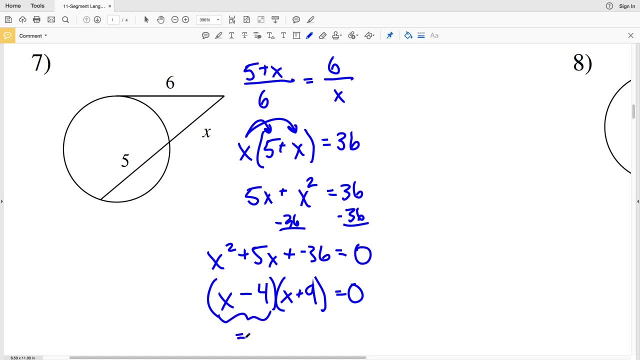 order to get that equal to 0. that means that X minus 4 equals 0 or X plus 9 equals 0. however, if X plus 9 is equal to 0, that means I'll have a negative 9, which I will not have a negative. 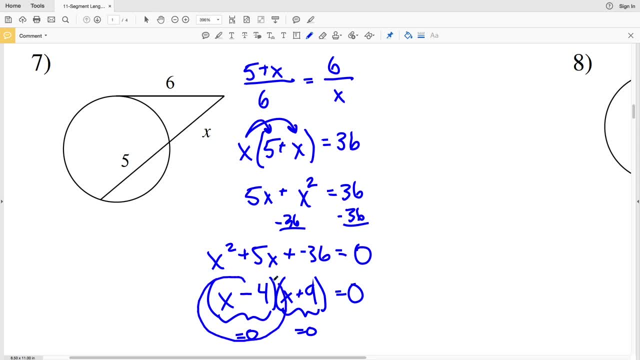 measurement for the lengths. so I'm going to be looking at X minus 4 equal to 0, and if X minus 4 equals 0, I'd simply add 4 to both sides to get that X was equal to 4 in number 7, so 4 is X in number 7. and lastly, on this worksheet I'll have number 8. 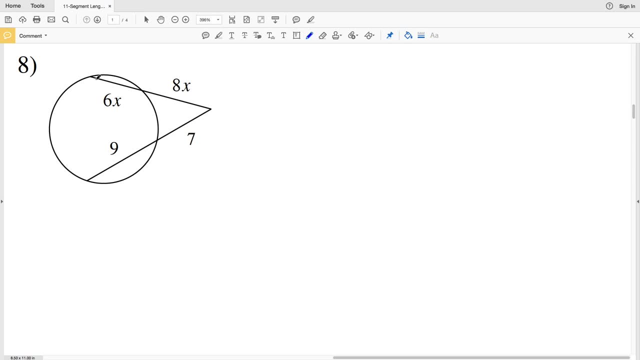 it's the intersection of secants. so the secant length including the cord, that entire secant length, 8 X plus 6 X. if we multiply that by the secant length without the cord- so excluding that cord- 8 X- that's going to be equal to the other secant length of. 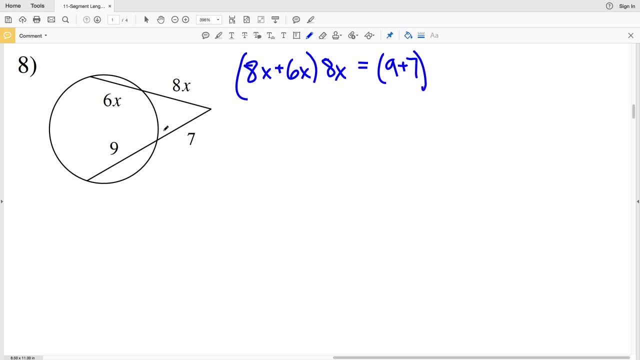 9 plus 7 times that secant length without the cord, which is 7. so, simplifying this problem, I'm going to need to distribute the 8 X 8 X times. 8 X is 64 X squared and I'm going to add that to 8 X times.